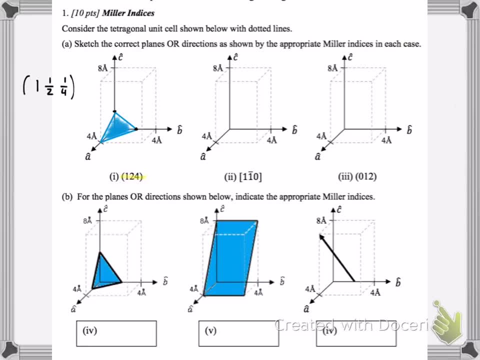 obviously is a section in a lattice Right. A lattice is a bunch of unit cells arranged together So you could reflect. Oh, I forgot to add these. So if you just want to put the intercepts there, One half B over two or C over 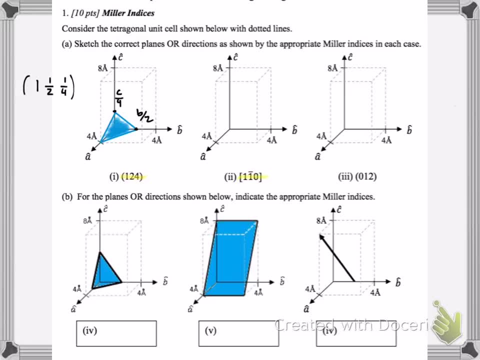 four, Simply just showing which point it is. Anyway, as I was saying, if you're going back to here, the unit cell has a ton of different local coordinate systems, you could say for each unit cell. So if we extend this coordinate system here we can draw our direction going. 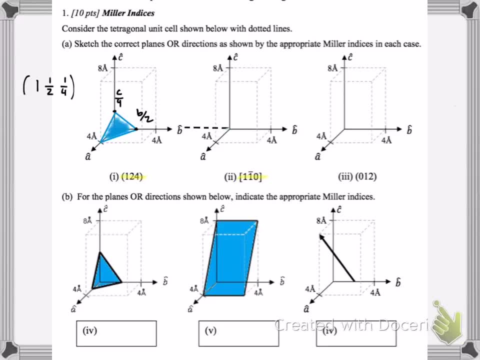 into that coordinate system to the left there. So we go one along A, But look, now we got negative in the B, So we have to go back in the negative direction of the B axis And then we don't move anywhere in C. So it's just like we move down in that direction. 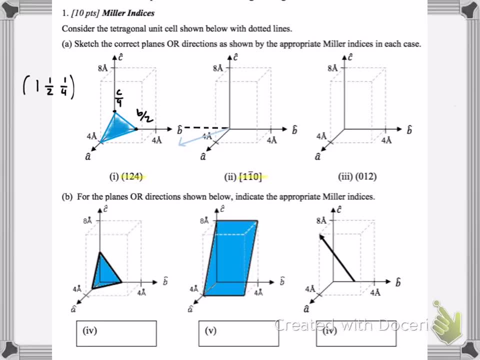 But how do we transfer that information into the unit cell? Well, it's simply, you simply shift it into your current coordinate system. So it looks something like that. So that's one way to look at these Miller indices is to expand your coordinate system and look at, instead of just the small one local coordinate system. Look at local. 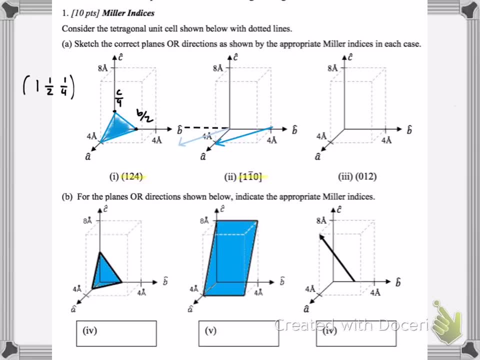 coordinate systems adjacent to your unit cell. Cool, So now we got another plain problem. So simply take the reciprocal. The reciprocal of zero, mathematically, is technically infinity, And we'll talk about what that means in a minute. Reciprocal of one is one. Reciprocal of two is one half. 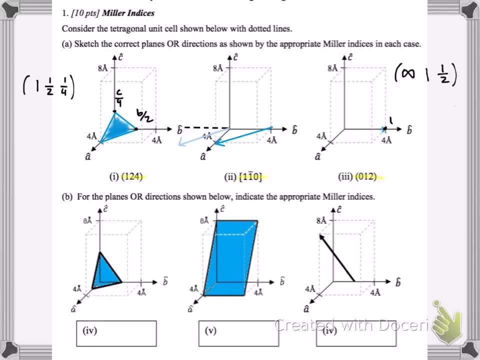 So the one there I should. I should explain what the infinity is. I wrote it somewhere, but it's not popping up. So the infinity pretty much means parallel to whichever axis the infinity is located. So in this case we need to be parallel to A, So we'll show you how to draw that in a minute. 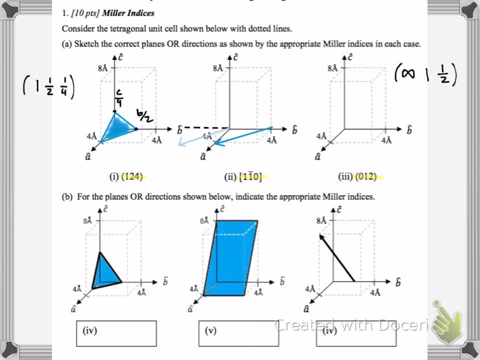 But notice, let's look at what we do know. So one One along the B axis. So we hit the B axis at one And we go half way up on C. Right, But we have to be parallel to A. So in order to be parallel to A, we have to draw our plain as such, And that's why 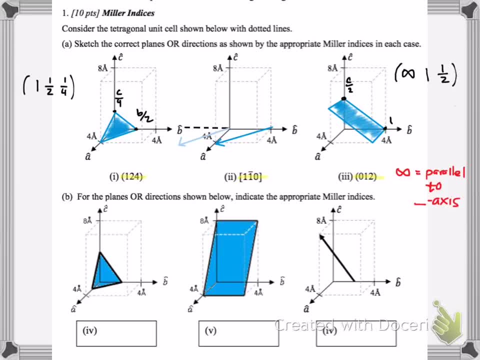 the infinity means parallel to the whichever axis- Cool. So notice how that part of the plain is always parallel to the A axis and it will never intersect it. Cool, Alright. Now let's look at part B, where we have to give the Miller indices. 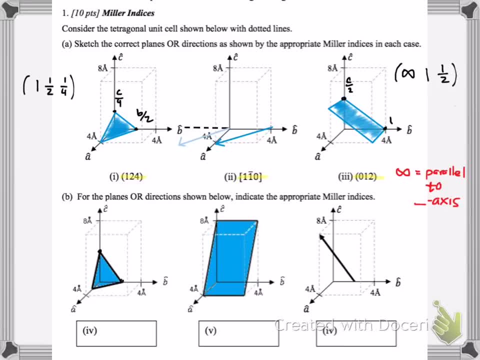 from the plains or directions shown. So let's look at the plain over here, Let's look at the intercepts there, So that looks like to be half way along B and half way up C and half way at A. If you just look at the unit set, it looks like half way. 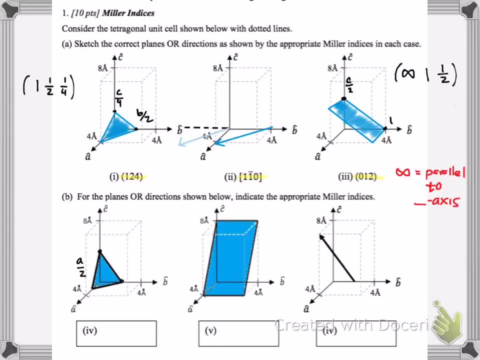 in every direction on each axis. So we got A over 2 here, We got B over 2 there and C over 2. Half way along up each axis. So simply how we would start off our Miller indices for indicating the plain is well, one half, one half, one half. 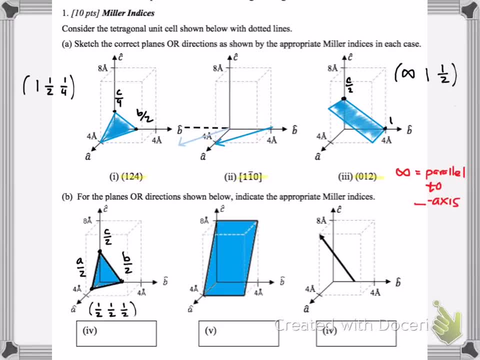 Right Went half way in each direction. But we know that plains for Miller indices cannot be or must be in integer notation. So, simply, what we do is we multiply or, excuse me, we take the reciprocal and doing that, we'll give 2,, 2,, 2.. Awesome. 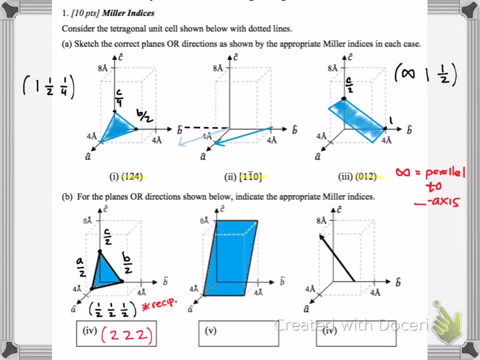 How do we? yeah, I won't go, That's a wrong mistake, I won't go there. Okay, Now let's check out this plain here. So how do we handle this one? Well, it hits the A axis right, exactly, and then it goes. 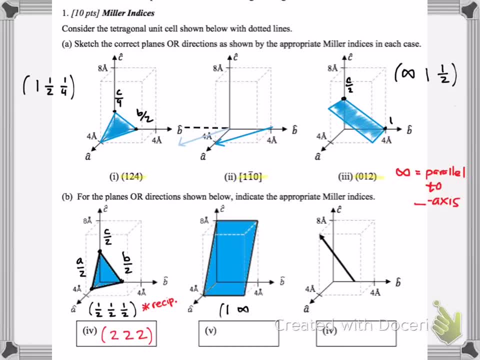 it's always parallel to B because it never intersects it and it hits the C axis. So how do we write that? Well, you'd have to take the reciprocal of that. So the reciprocal of 1 is just 1.. The reciprocal, technically, of infinity is 0, and then we have reciprocal of 1 is 1.. 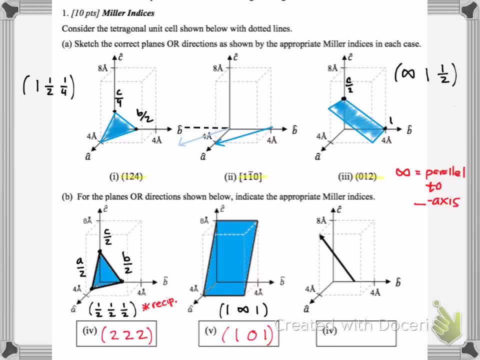 And the reason you knew to put infinity for the second coordinate is because it's not touching the B axis at all. It's always parallel, It will never intersect it Cool Next direction. So simply, you know, see how far you go, So how far. 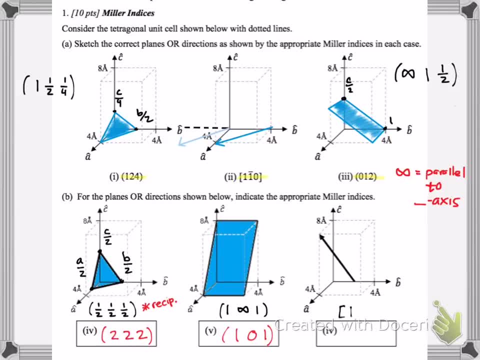 do we go for pointing this direction here? Well, we go 1 along A, since we're on the upper left corner, So we're at the corner on the A axis, And then we go 1 half in the negative B direction, because notice how it's coming out. 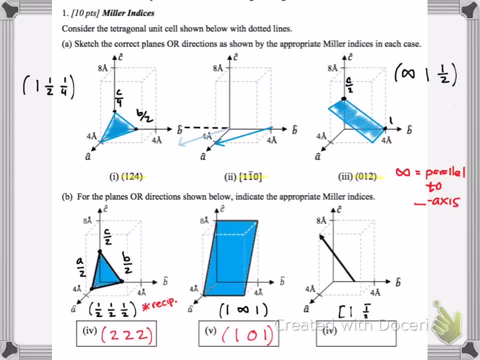 It's similar to the second problem in part A, where you have to draw that adjacent unit cell. But I forgot to draw that for you all And then you're going to go up in C. So had the 1 half not have been negative, it would have been pointing in another.